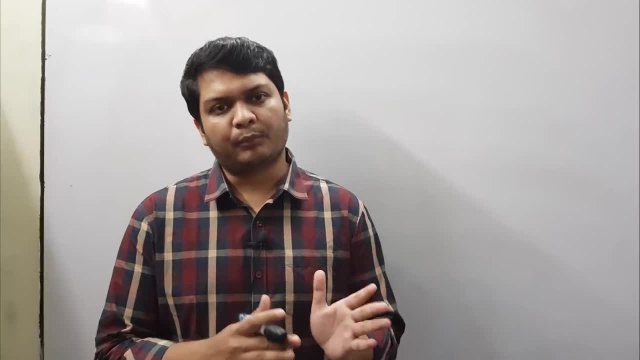 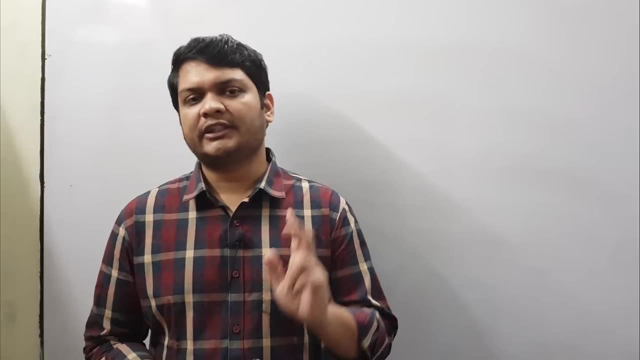 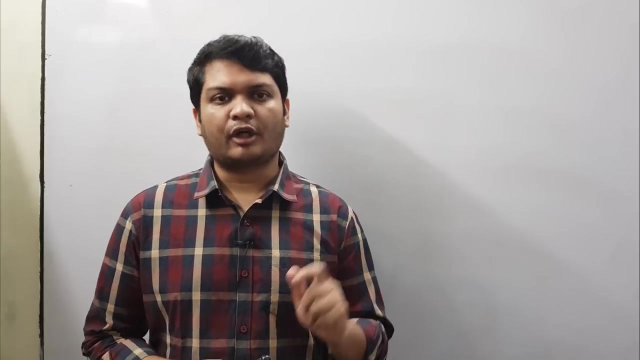 Say, a function is something which takes some inputs and gives you some corresponding outputs, to say the least and in an easy manner. And a function has two conditions. The first condition is that each and every input of the function must have a corresponding output. Second condition is: 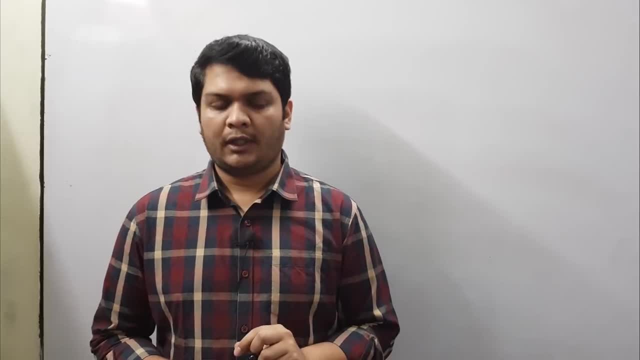 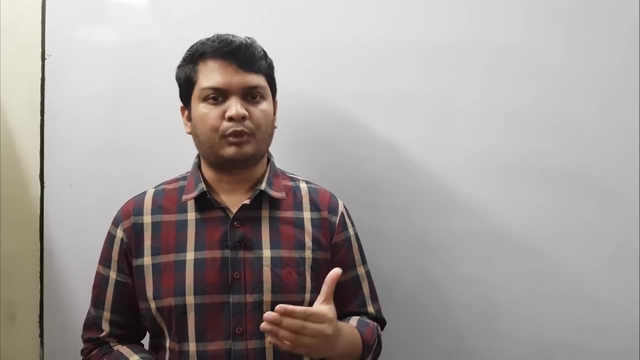 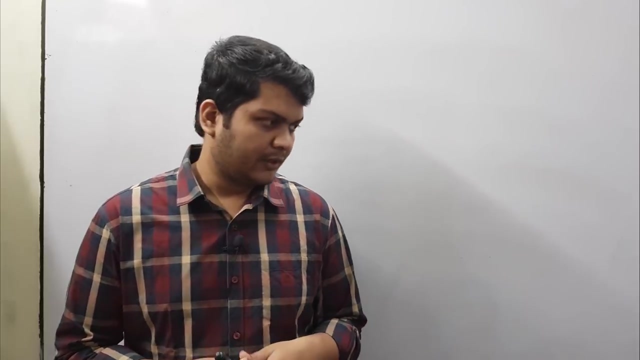 that no input can have more than one output. So today we'll be focusing more on the first condition, which says that each and every input must have an output, Otherwise we cannot call that function as a function, So that will be not a function. So if we look into this function, say 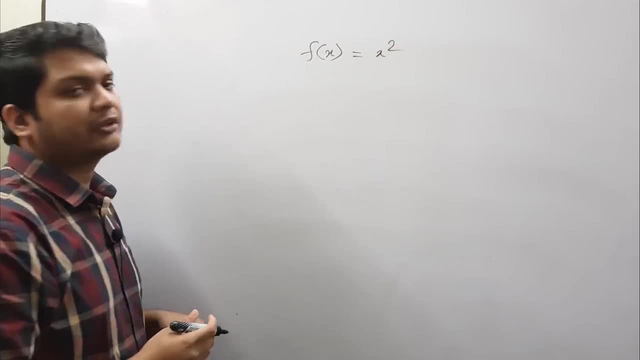 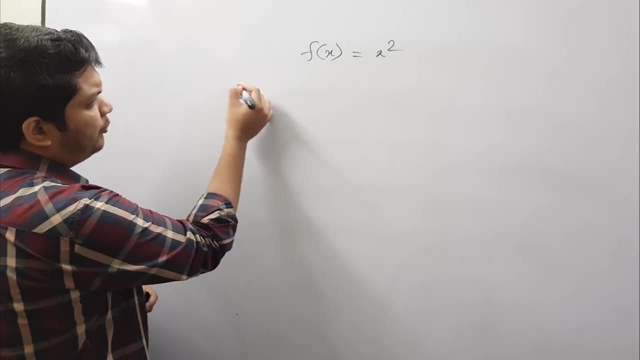 for example, f of x equals to x square. We'll be trying to put some different values of x and we'll see whether we're getting some outputs or not. Say, if we put x equals to 1, then f of x equals to 1 square. 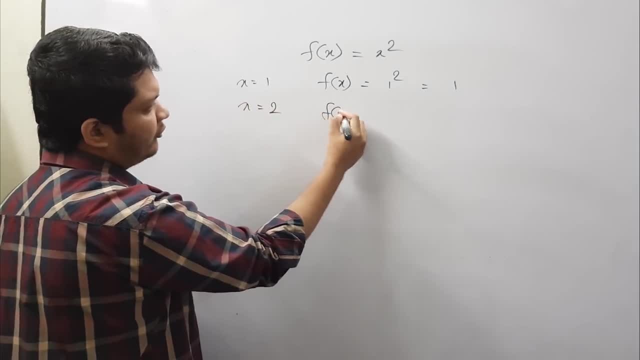 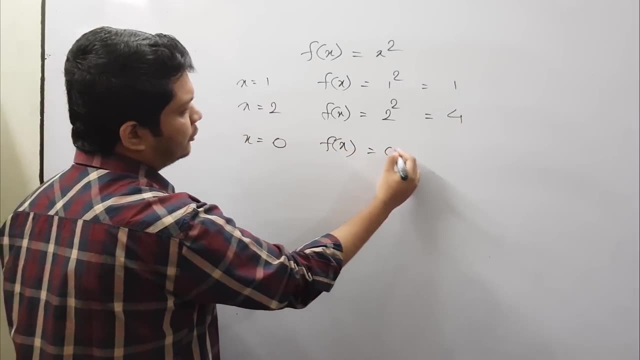 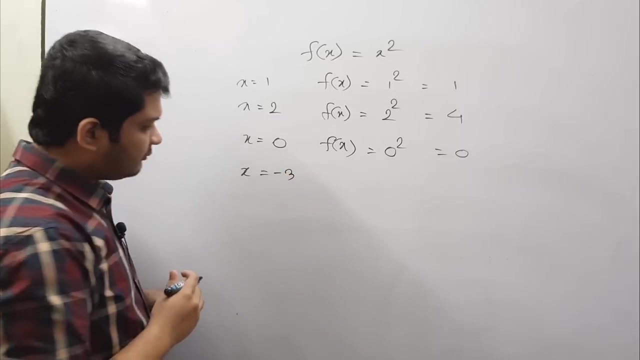 equal to 1.. If we put x equal to 2, f of x equals to 2, square equal to 4.. If we put x equal to 0, f of x equal to 0, square equal to 0.. If we put some negative values as well, So say we are putting x. 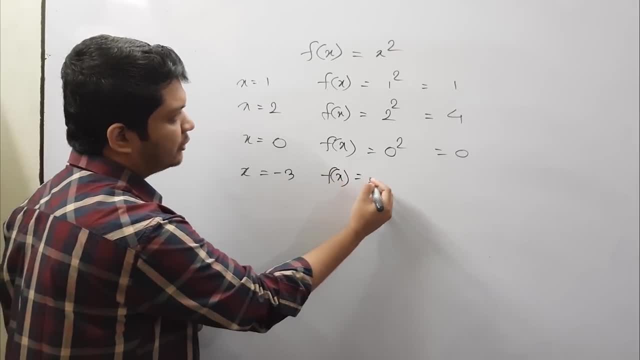 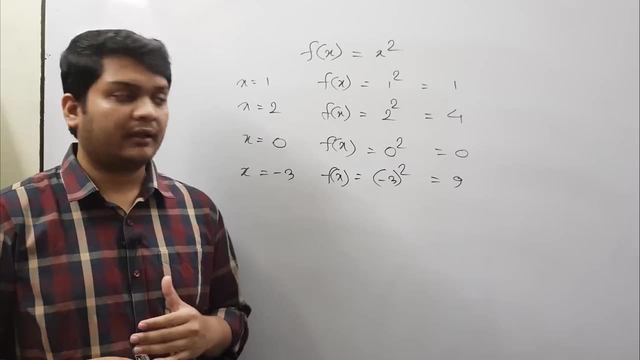 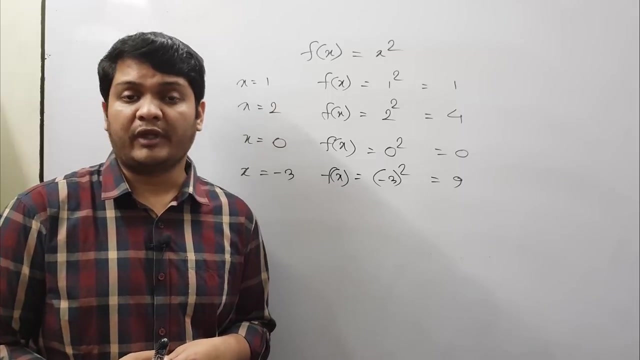 equals to minus 3, then f of x equals to minus 3, square equals to 9.. So we can see that in this way we'll get outputs for each and every values of x, So, which satisfies the first condition of function, that we are getting corresponding outputs for each and every inputs. So 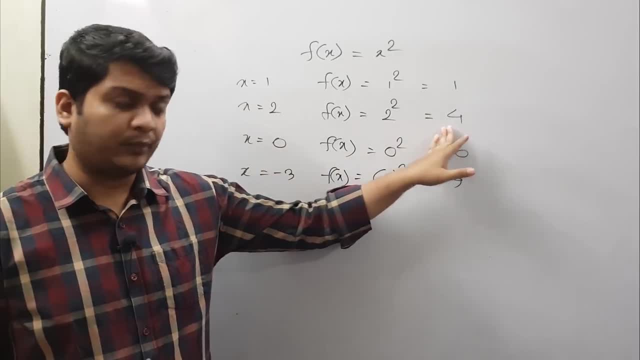 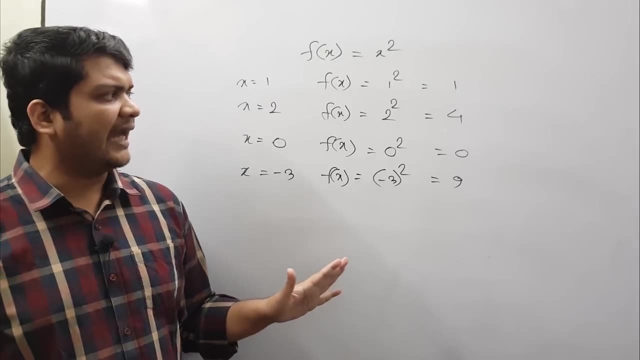 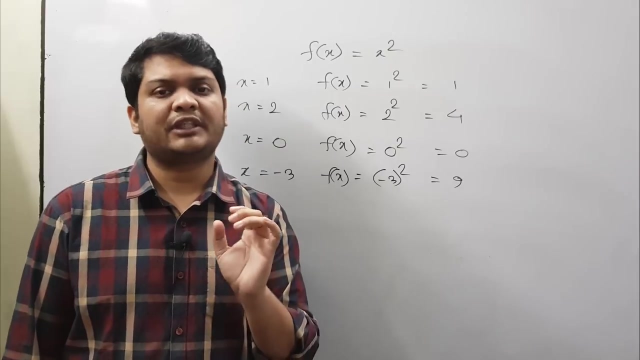 we can see that for values greater than 0, we are getting outputs. for the values of 0 and less than 0, we are also getting outputs, And in this way we can see that for each values of x, we are getting some outputs. So this is a function, But sometimes there will be some situations when 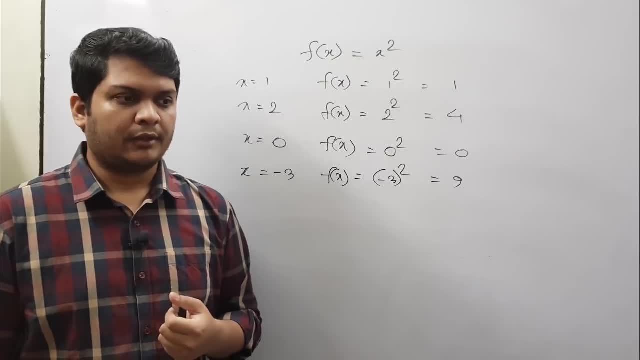 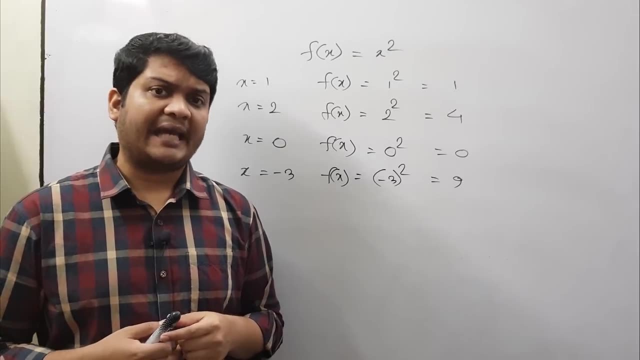 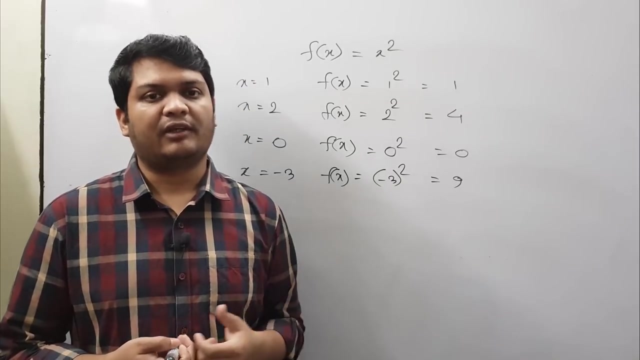 we'll see that we are not getting outputs. So in those situations, what would we do? whether we will be canceling those terms as functions, or whether we'll try to find some way to calculate those values. So let's see what we have. 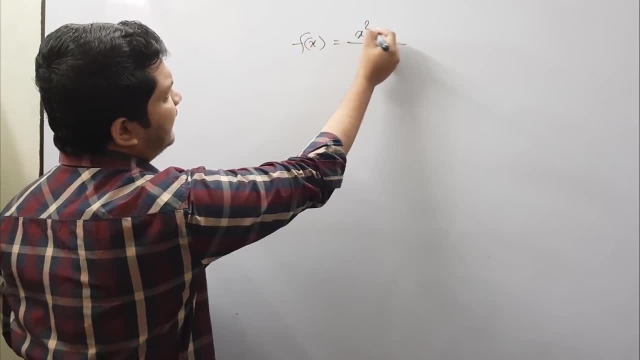 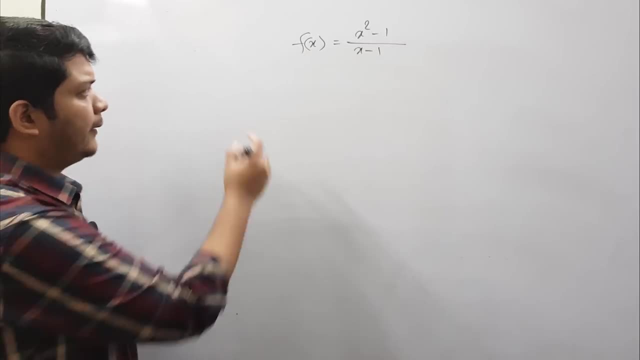 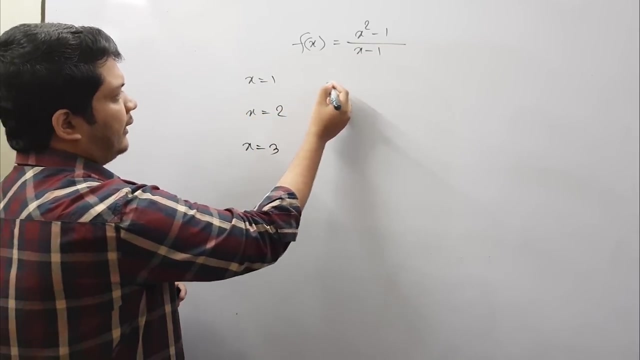 Say we have a function: f of x equals to x square minus 1 divided by x minus 1.. So let's get started with some values. say x equals to 1, x equals to 2, x equals to 3, f of x equals 2, f of x equals 2, f of x equals 2.. If we put x, 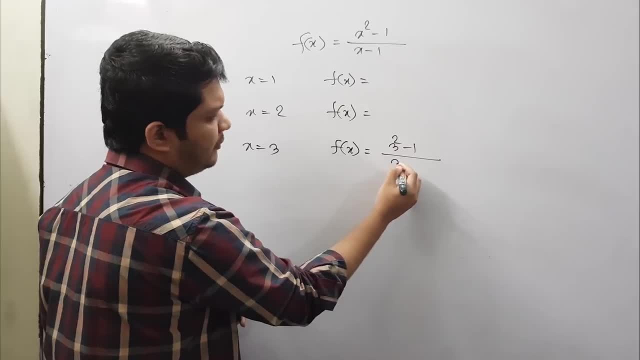 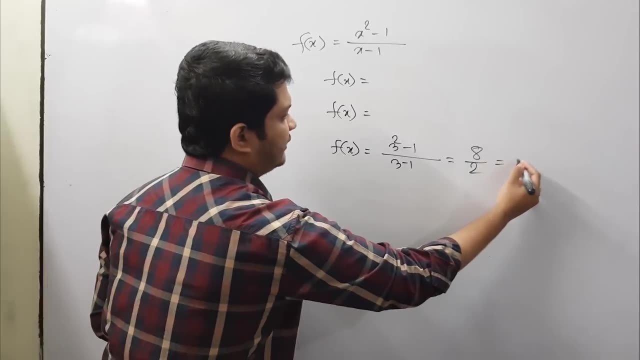 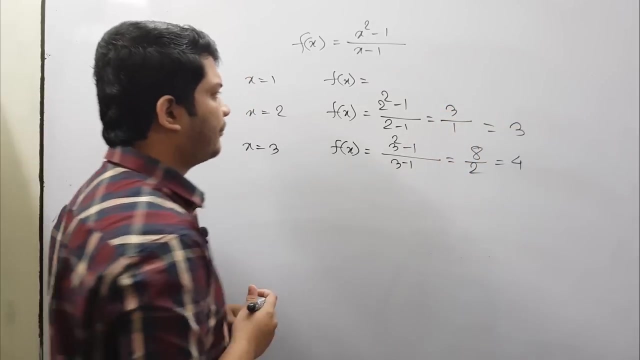 equals to 3, we will get 3 square minus 1 divided by 3 minus 1, which is equal to 3 square minus 9 minus 1, divided by 2.. So this is equal to 4, and this is 2 square minus 1 divided by 2 minus 1, which is 3, divided by 1, which is 3.. But 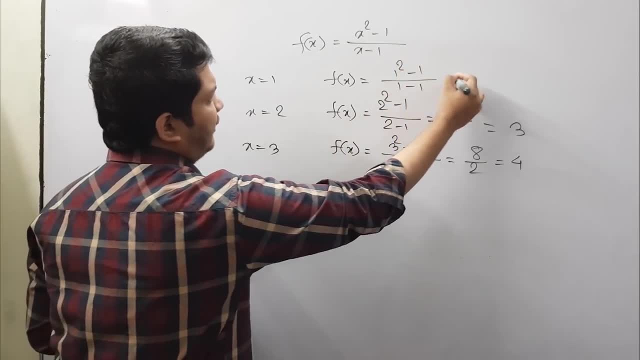 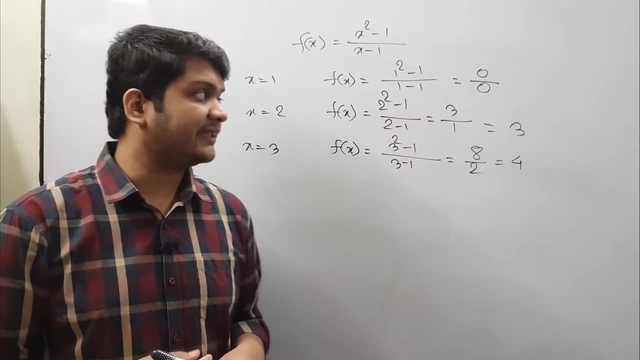 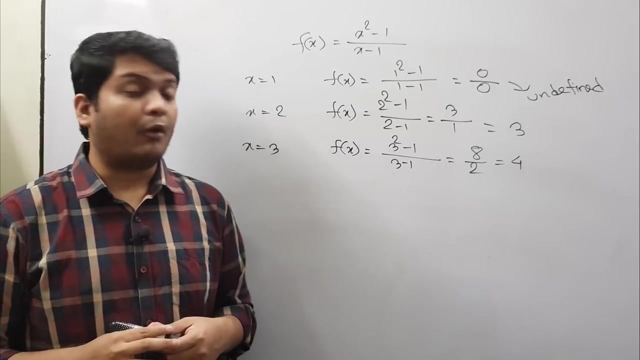 here we will see that 1 square minus 1 divided by 1 minus 1, resulting in 0 divided by 0, and we know that 0 divided by 0 this is undefined, So what will we do now? We are not getting any outputs for the input x. 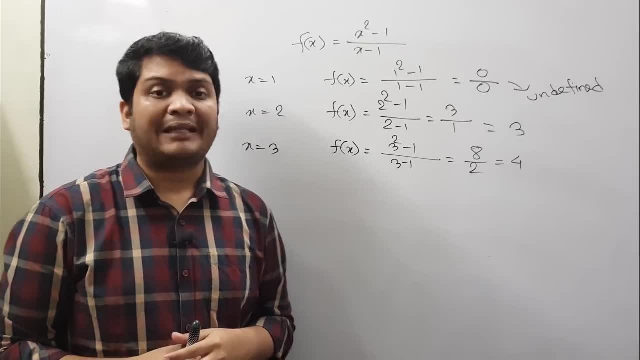 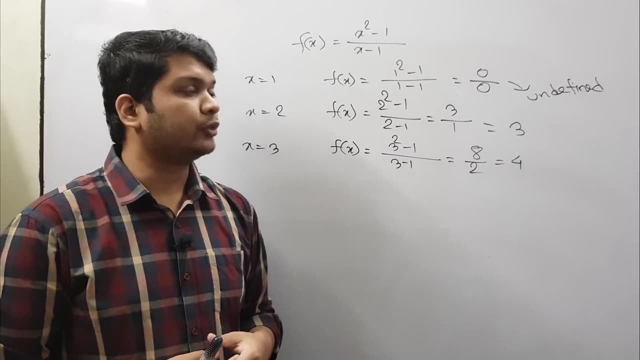 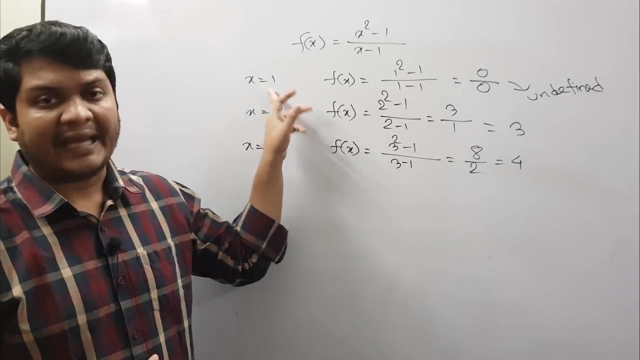 equals to 1.. So mathematicians somehow found a way to calculate this value, and we will be now looking into that procedure. So what is that procedure? The procedure that we are not being able to put the values of x equals to 1.. So we'll. 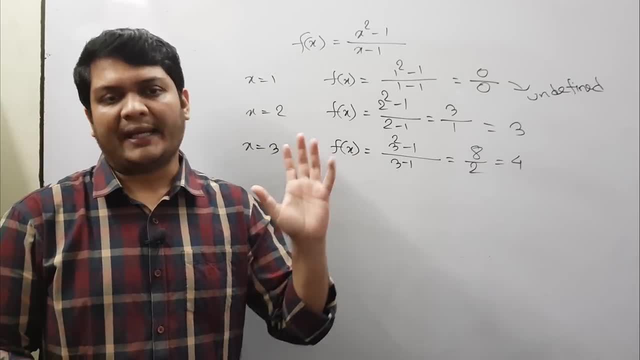 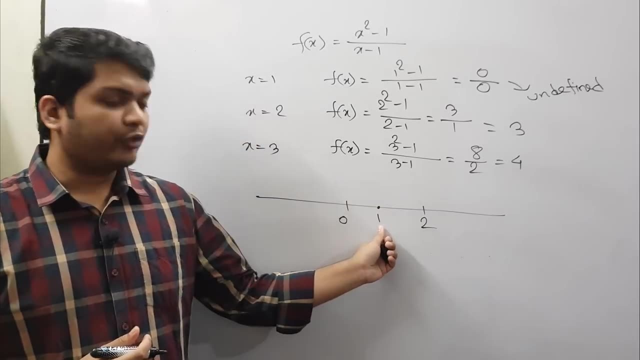 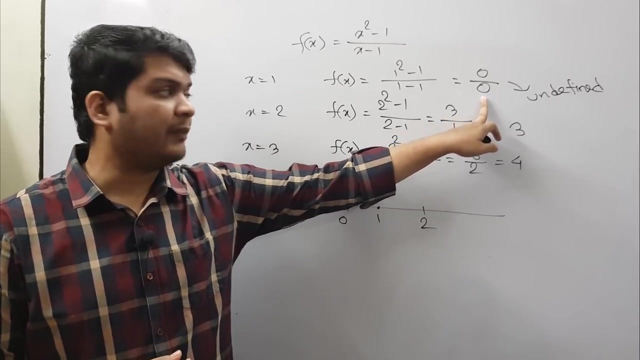 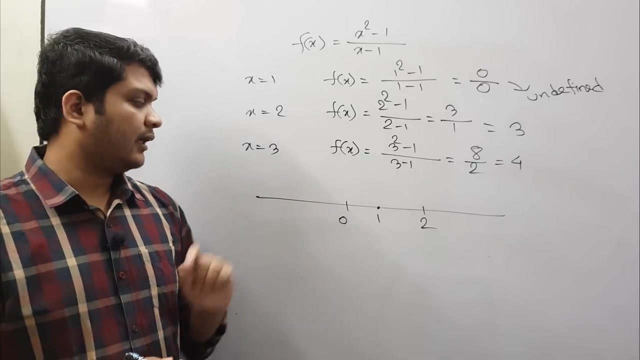 try to put values which are close to 1.. What do I mean by that is, if we put 1, we are getting some problems, that we are getting results as 0 divided by 0, which is undefined. So we will give values which are much more closer to 1.. So when we say we will put values closer to 1, we 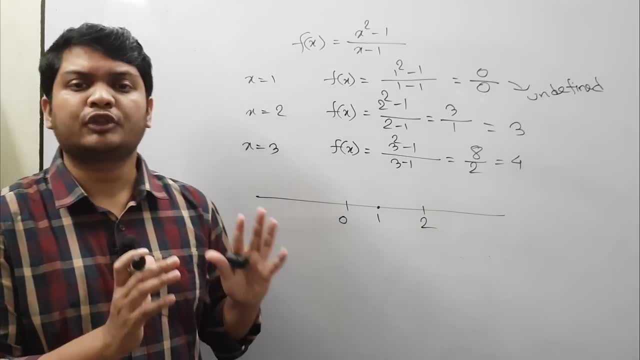 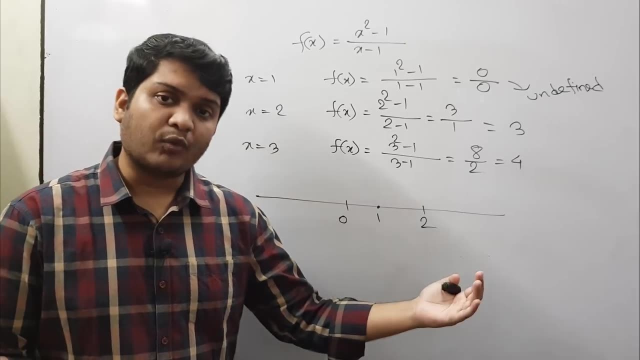 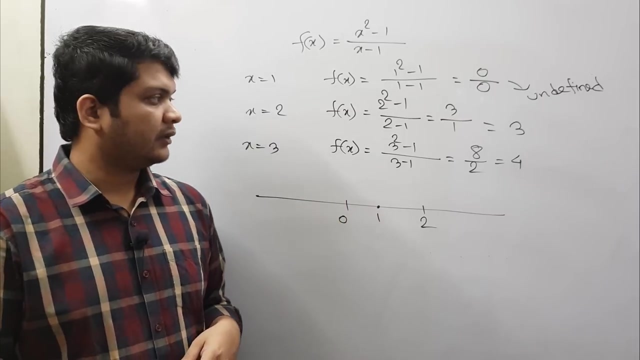 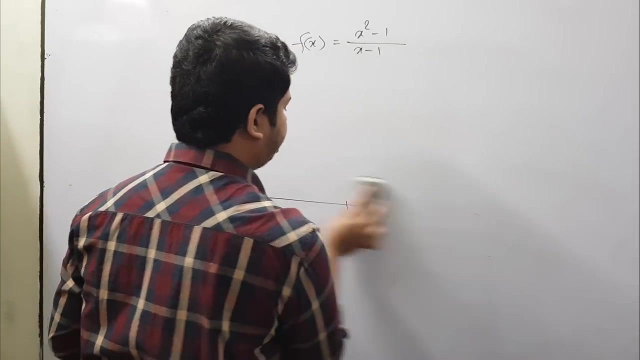 have two options. We can either start with values which are less than or greater than 1 and then gradually increase, or we can start with values which are greater than 1 and gradually decrease. So we'll have two different ways to calculate the values. So let's see how it would work. 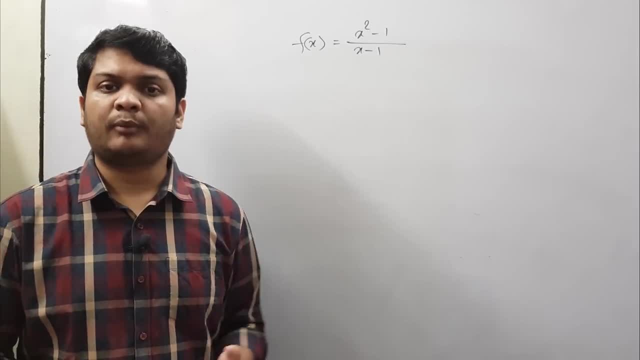 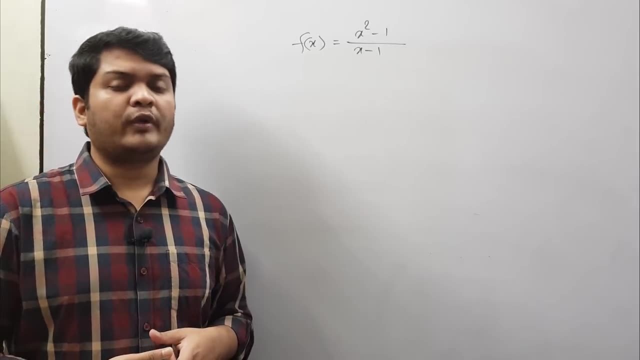 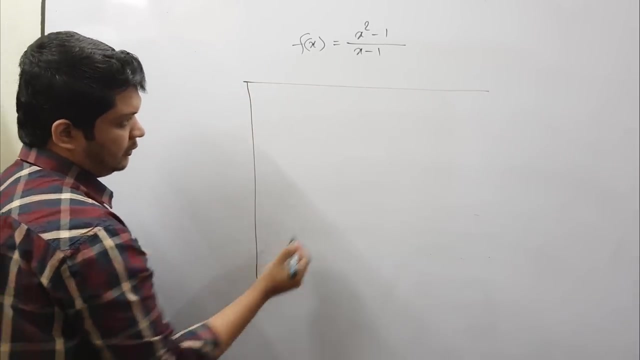 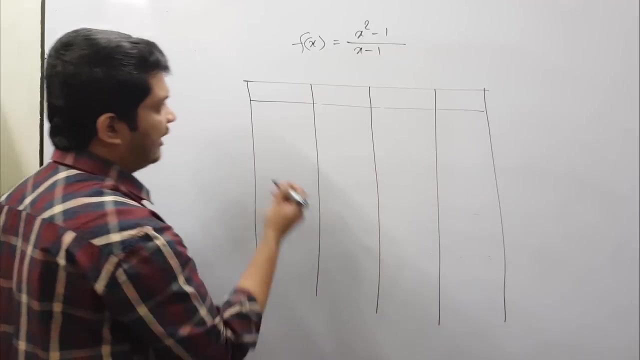 As we have already seen that we can move towards 1 from two different directions, whether we might try from values less than 0, or we can start from values greater than 1 and gradually decrease. So let me draw a box and calculate the corresponding values. 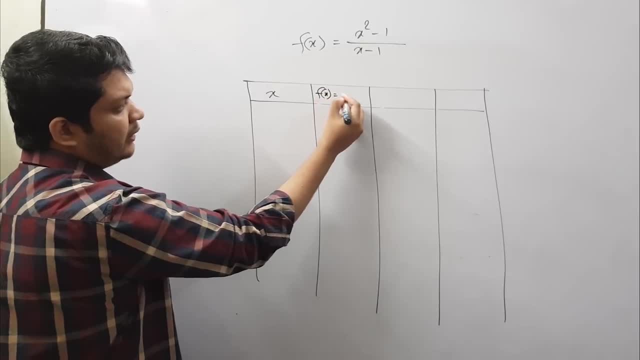 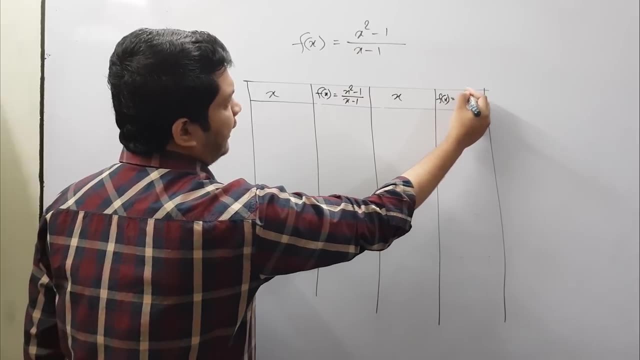 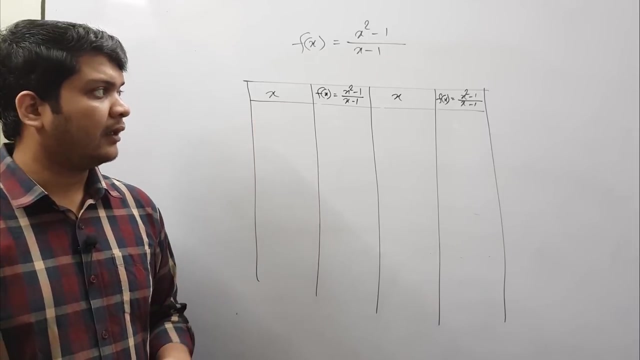 Here I'm writing x and this is f of x equals to x square minus 1 divided by x minus 1.. Again, x and f of x equals to x square minus 1 divided by x minus 1.. So I want the values of x and x square minus 1 to be 2 with respect to trying to calculate. 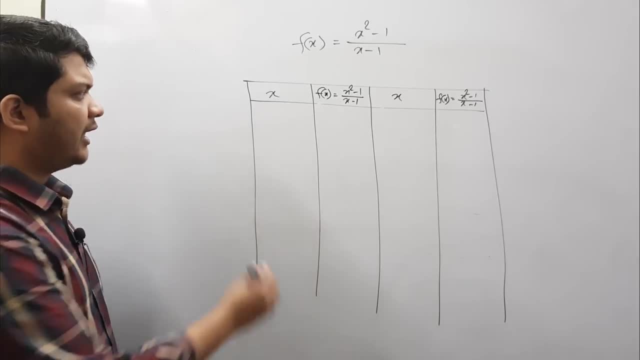 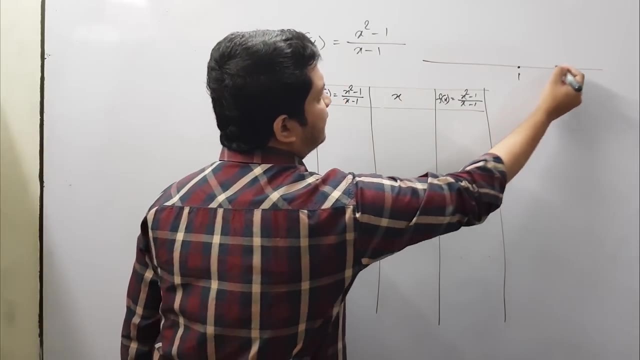 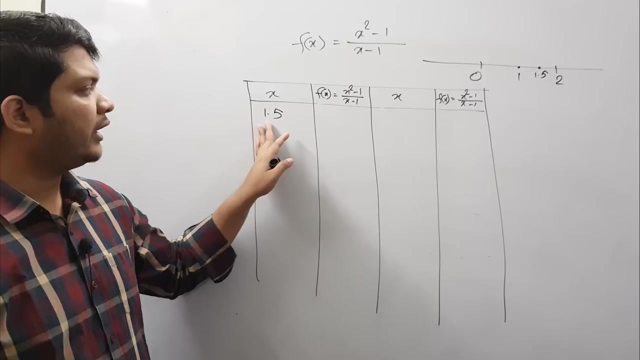 x. We are putting our value x, says its message from f, butwa will give us xF of x, which is x by 1 equals pozyminus 1 divided by x minus 1.. Here we will be starting from values which are greater than 1 and gradually decrease. Say we are putting values: x equals to 1.5.. If we look and into the number line, you can see that 1.5 is somewhat closer to 1. so we are putting the values 1.5 and we'll be putting different values. We'll be putting values 1.5 and we'll be putting different values- 2, so they willunt at the same time. 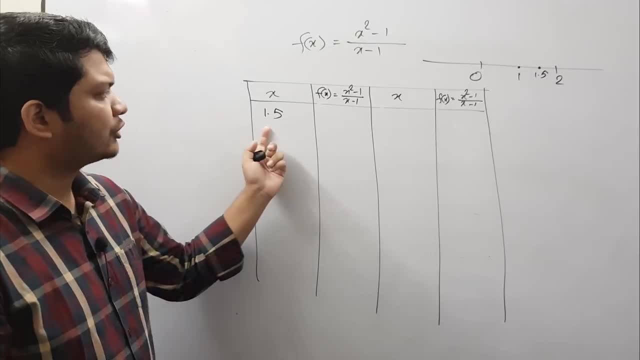 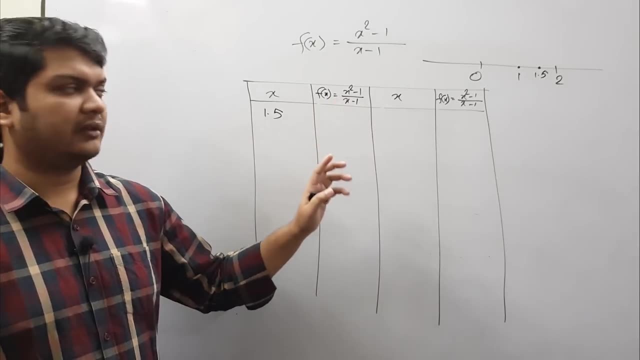 will be much more closer to 1.. So when we put x equals to 1.5. if we calculate the values of f of x, we'll see that 1.5 square minus 1 divided by x minus 1, that is 1.5 minus 1 and 1.5 square minus. 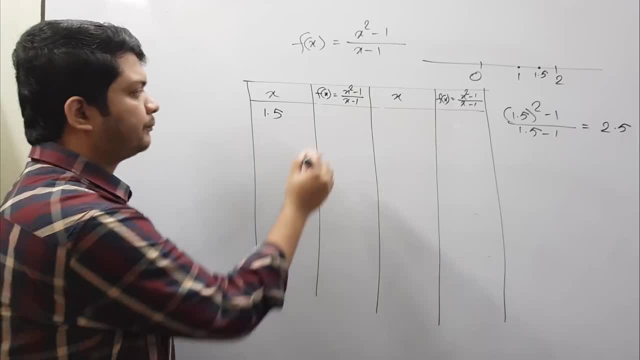 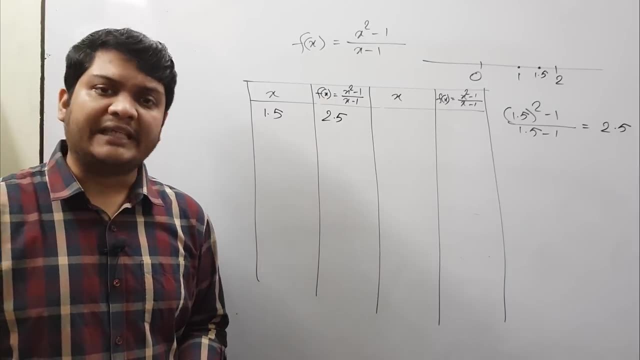 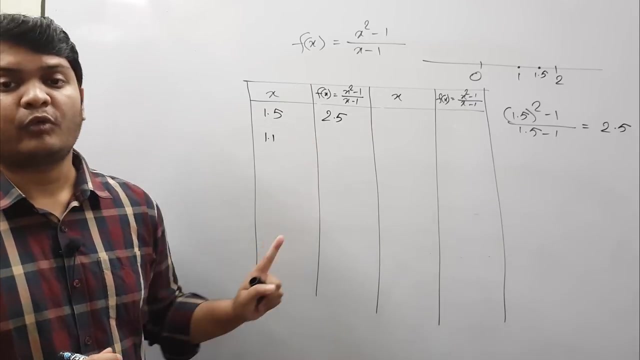 1 will get the result as 2.5.. So you can see that we are getting some values for 1.5.. So let's see if we get much more closer what happens. So let's put the value 1.1.. As you can see, 1.1 is much more. 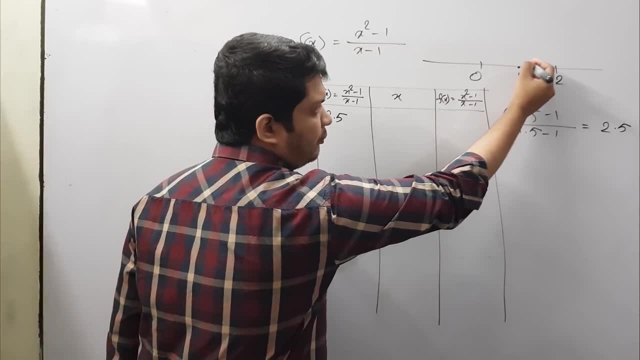 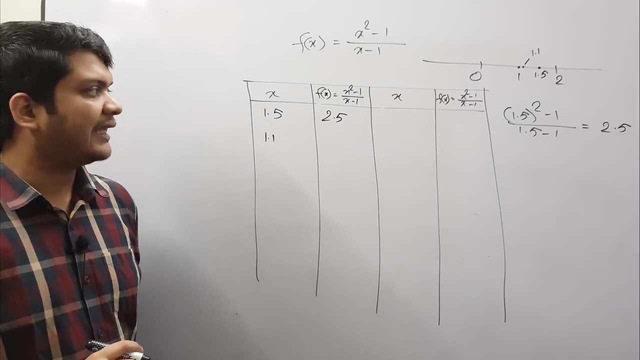 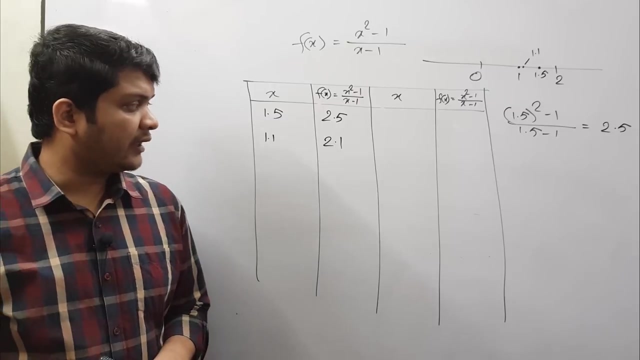 closer to 1, right. We'll be putting this value somewhat closer to 1, right, okay? So 1.1 will give 1.1 square minus 1, divided by 1.1 minus 1, and you will get the result 2.1.. If you have calculator, 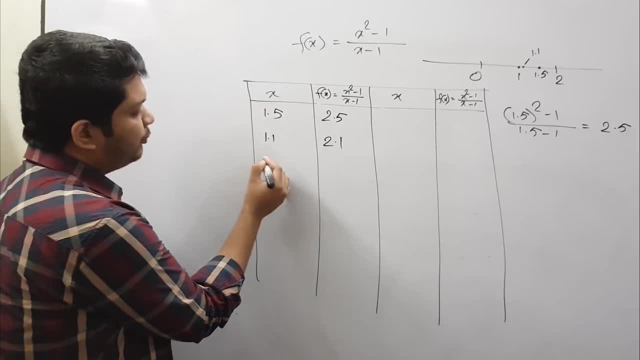 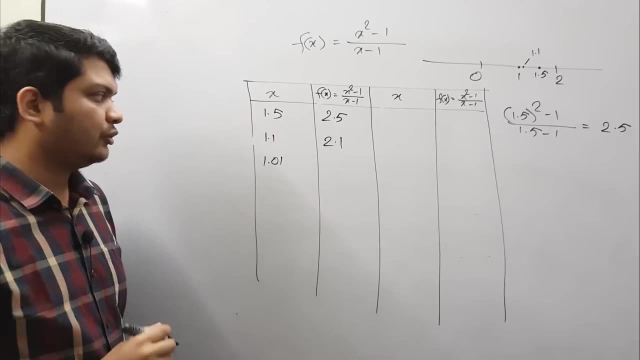 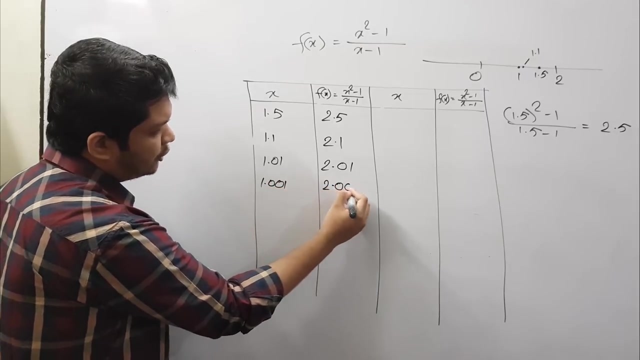 around you. you can calculate these values Again. if you put 1.01, which is much more closer to 1 than the upper two values, we will be getting as 2.01.. If we put 1.001, we will get 2.001.. You can calculate this value. I have calculated earlier. 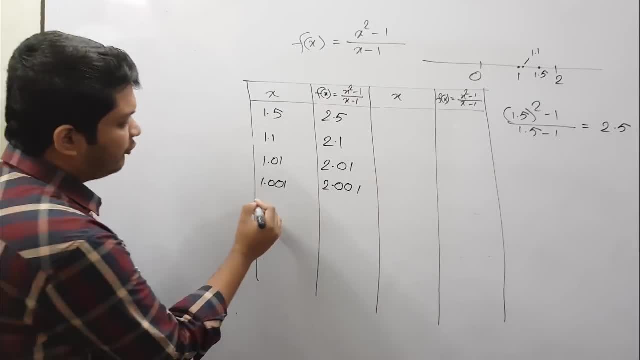 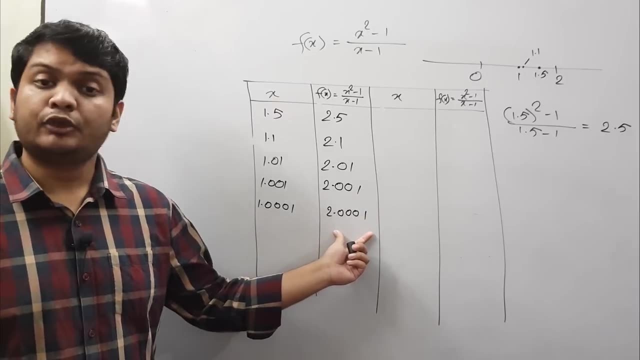 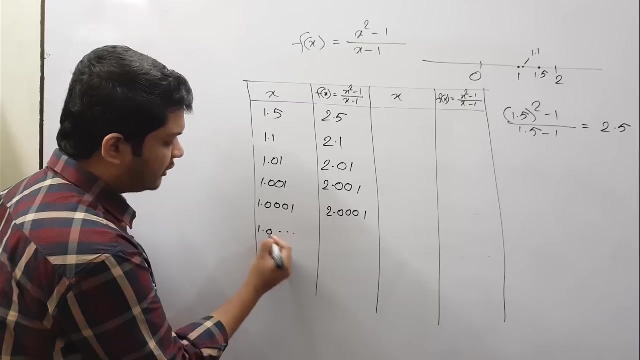 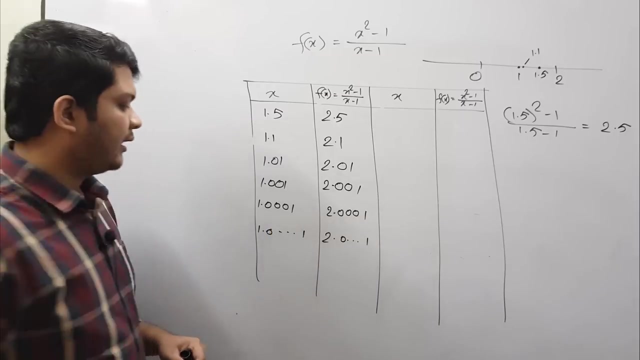 so I am not writing each and every values In this way. if we increase the number of zeros, we'll see that the result is approaching towards 2.. Because if we put one point- infinite number of zeros- and then a 1 say 0.1, we'll get the result as 2.0.1.. So here, infinite number of. 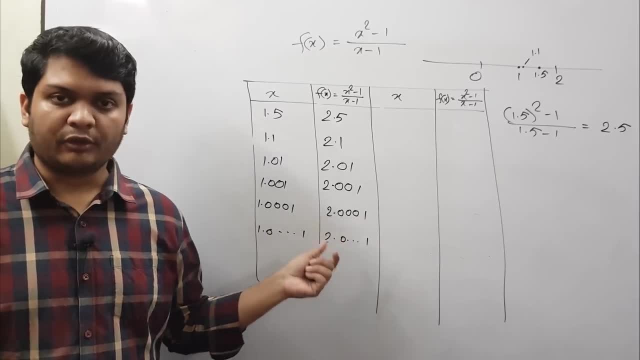 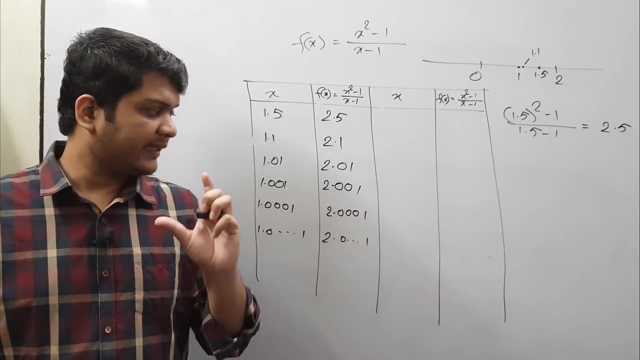 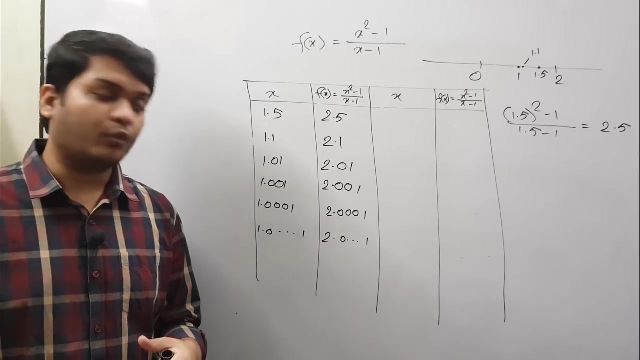 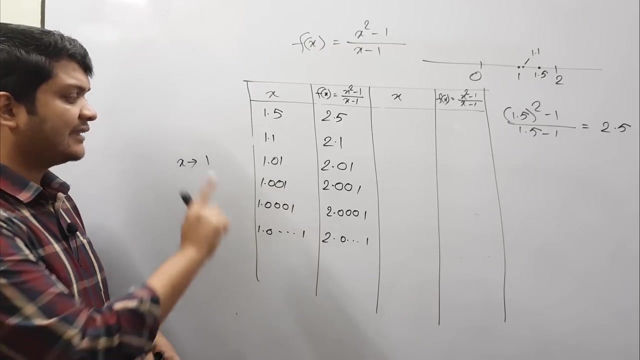 zeros, and we'll see that this is 2.000. in this way, infinite number of zeros followed by 1.. So we can decide now that this value is approaching towards 1.. In mathematics we say that x tends to 1.. That is, the values of x is approaching towards 1.. 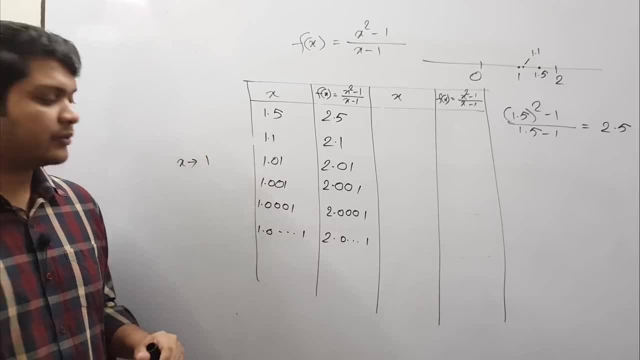 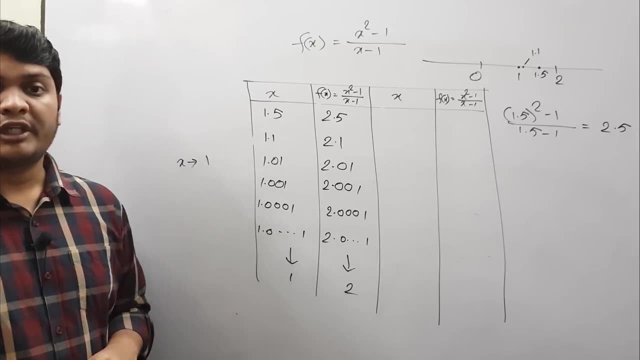 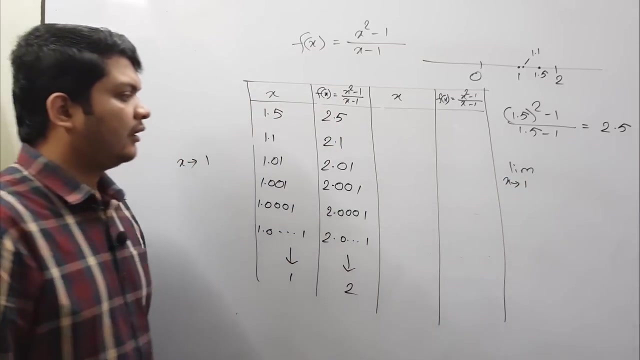 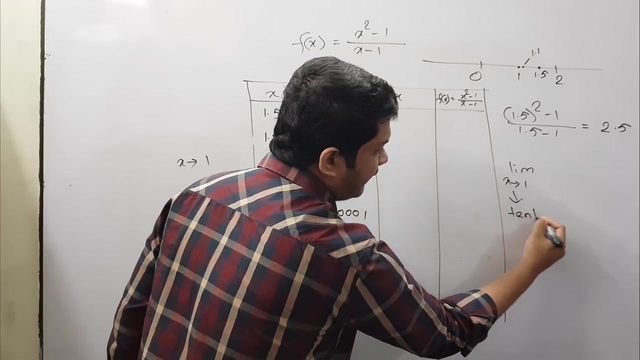 And what is happening to the output? the output is moving towards 2.. And this is moving towards 1.. In mathematics we call this procedure as limit that if we can put values which are closer to 1, 1,, that is, x tends to 1,. this sign is called tends to. As we can see, x is approaching towards 1.. 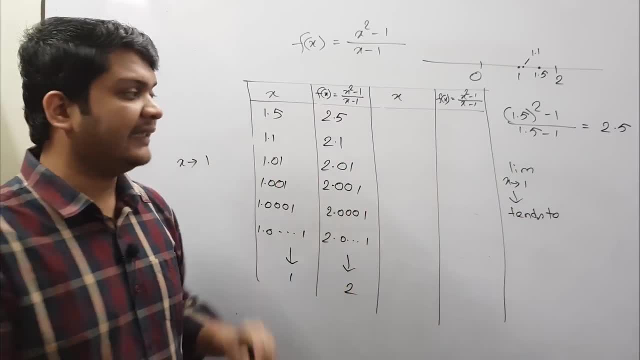 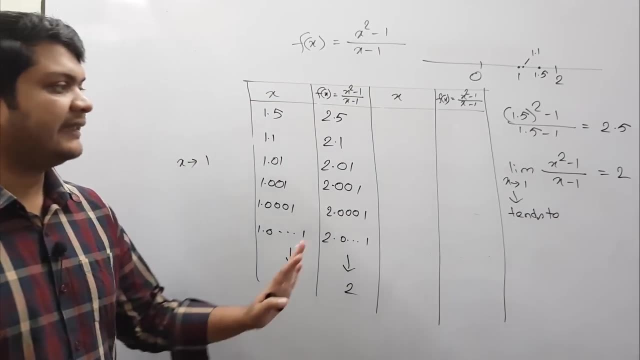 So we say that x tends to 1.. In that case, the values of the function x square minus 1, divided by x minus 1, will be equal to 2.. This is the concept of limit. So in short, we can say that: 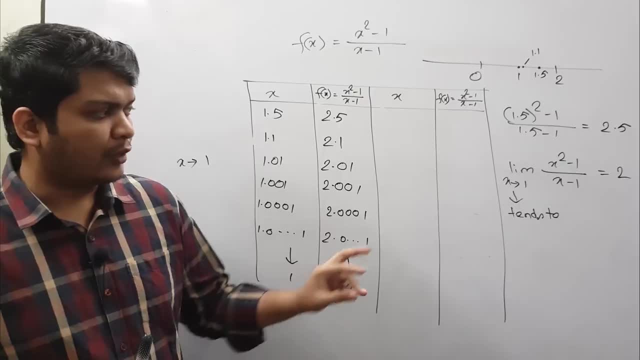 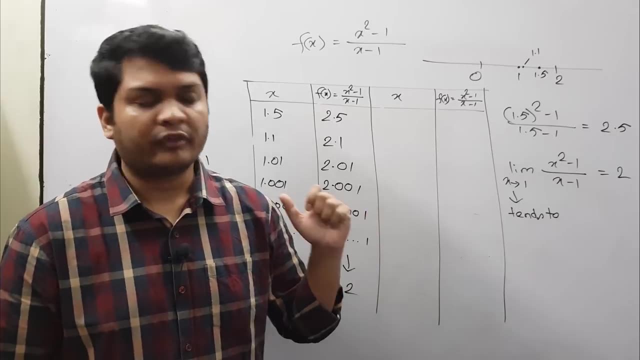 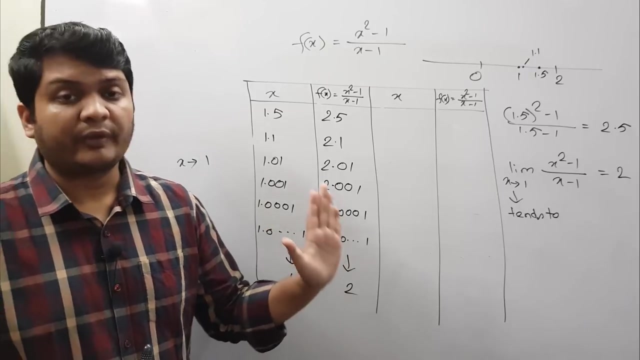 if we are being able to put the value as 1 or much more closer to 1, we will be getting the output as 2.. This is the concept of limit. So this was one part of the idea that we approached from values greater than 1 and gradually decreased the values. Now we will see from the other end. 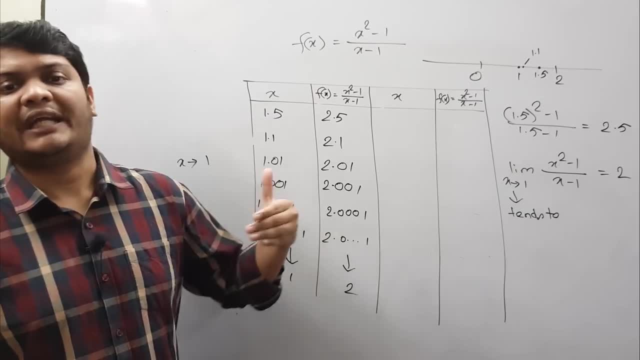 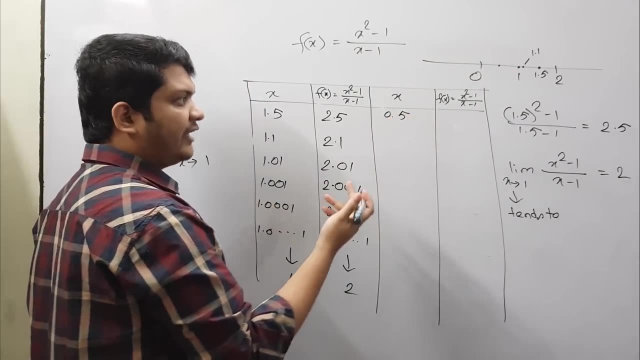 We will be starting from values less than 1 and gradually increase the values. Say, for example, x equal to 1.. 0.5, then if we put 0.5 square minus 1, divided by 0.5 minus 1, you will get 1.5.. If we put the: 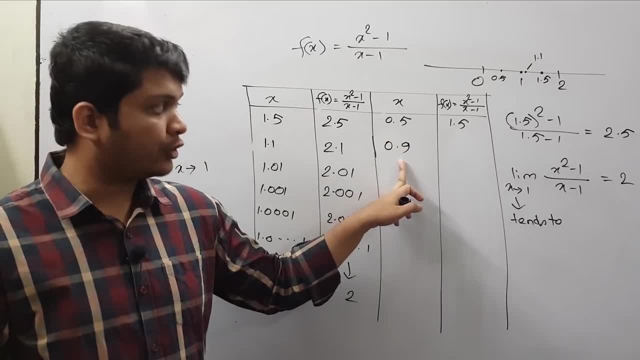 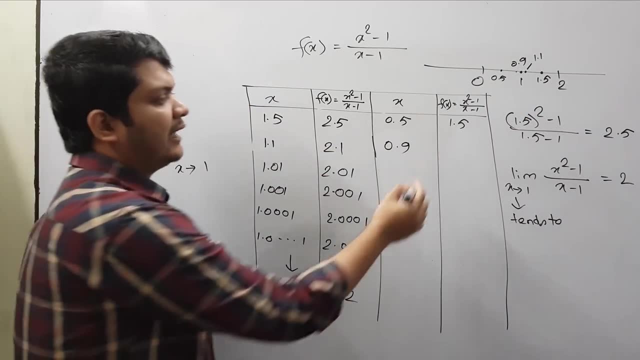 value 0.9,, which is much more closer to 1 than 0.5,, as you can see that this will be 0.9,, which is much more closer to 1, then we will get the output as 1.9.. And if we put 0.99, we will get. 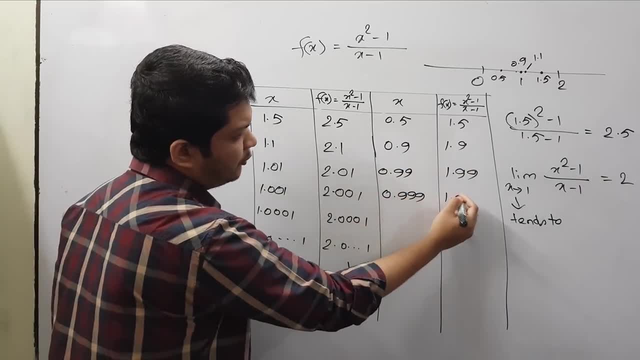 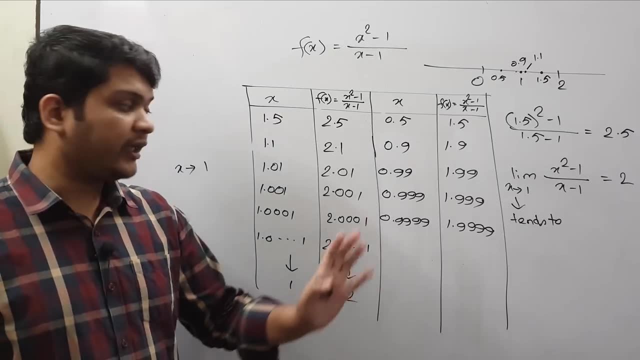 1.99.. If we put 0.999,, we will get 1.999.. 0.99,, we will get 1.999.. So in this way we can see that if we increase the number of 9s, that is, if you put 0.9 and 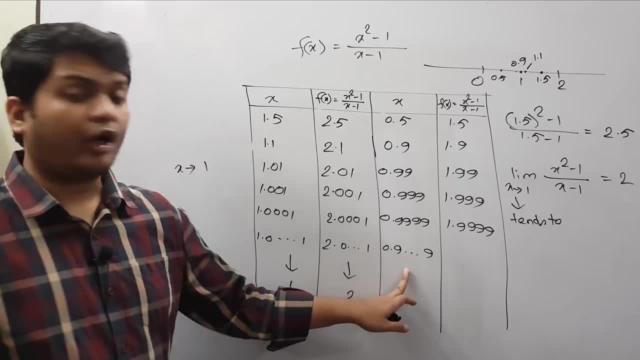 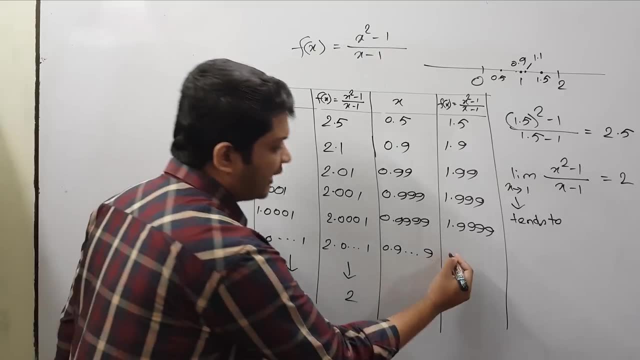 infinite number of 9s followed by 9,, which is almost 1.. I will show you in another video that this is almost equals to 1.. Then we will get 1.99.9.. So we can see that these values are. 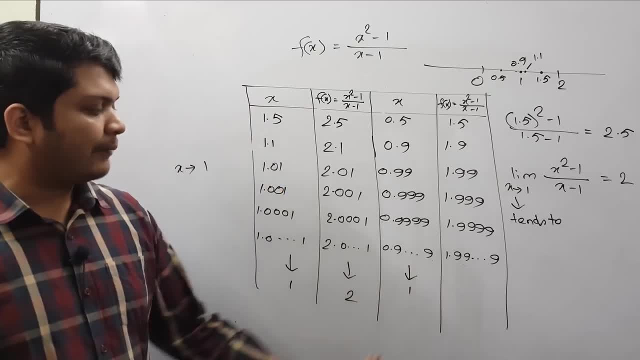 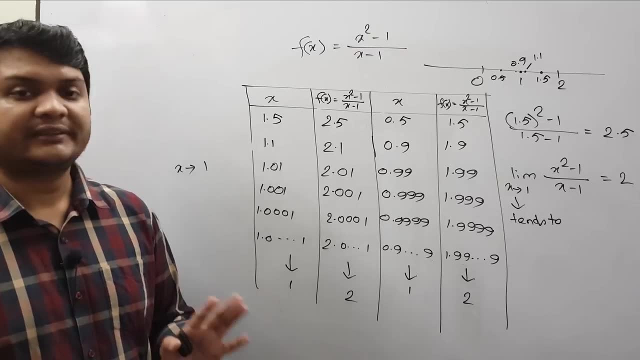 approaching towards 1.. So if we approach this value, we will get 1.99.9.. So if we approach this towards 1, the result is approaching towards 2.. So in both cases we have seen that if we start, 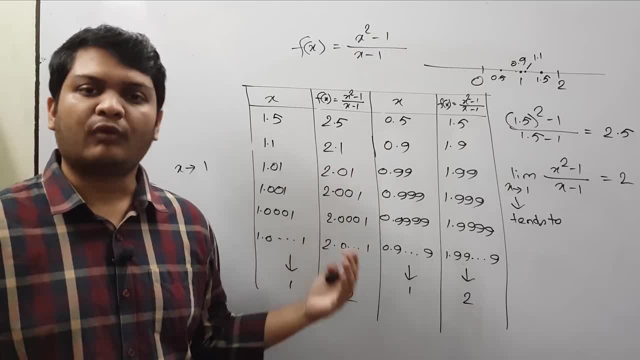 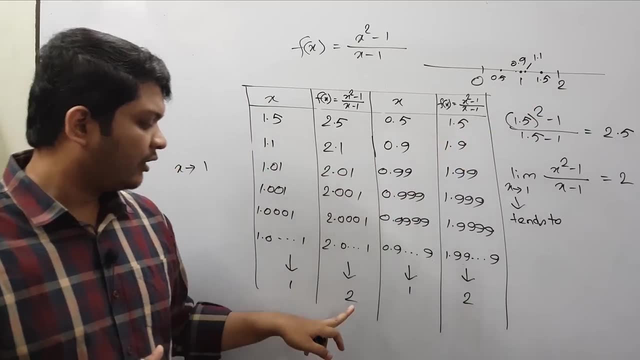 from either direction: if we start from values less than 1 and gradually increase the values, and if we start from values greater than 2 and gradually decrease the values. in either case, we are getting the result as 2.. So we can finally decide that the result must be 2.. Because in this 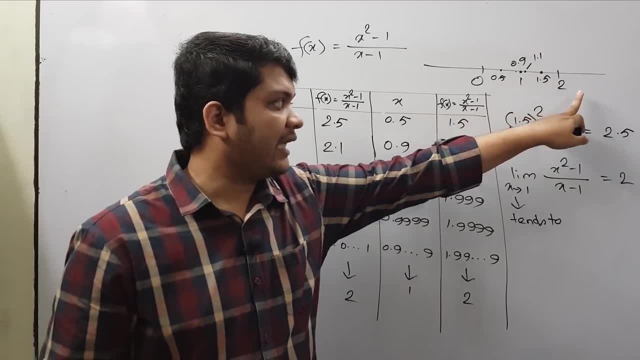 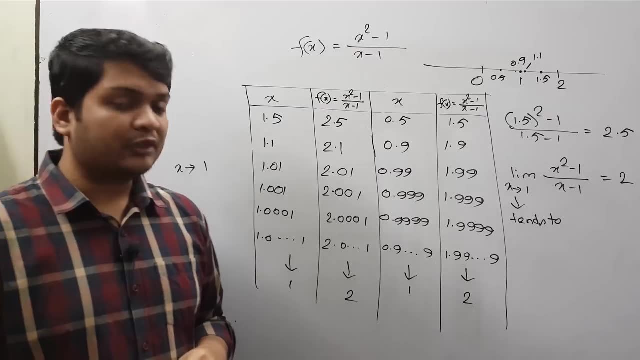 way we are approaching towards 1, we are getting 2.. Again, if we approach this way, we are also getting 2.. So the final result must be 2.. This is what we say in limit, that if x approaches or 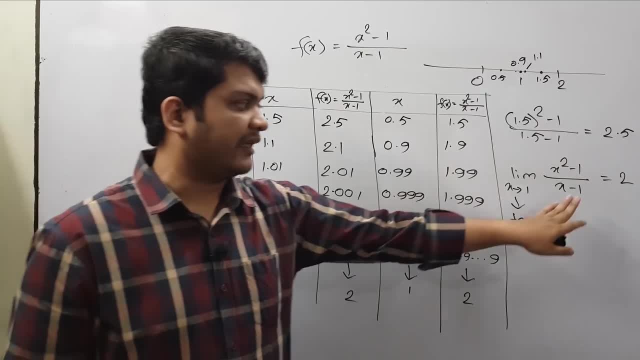 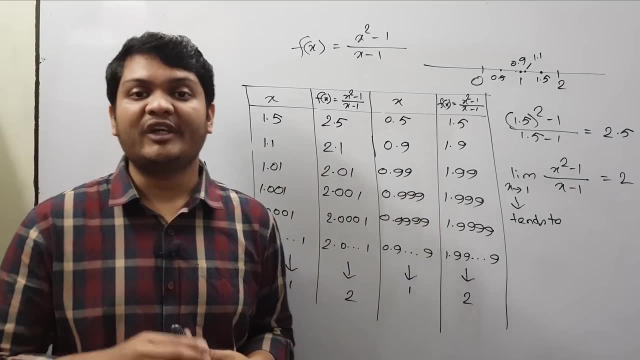 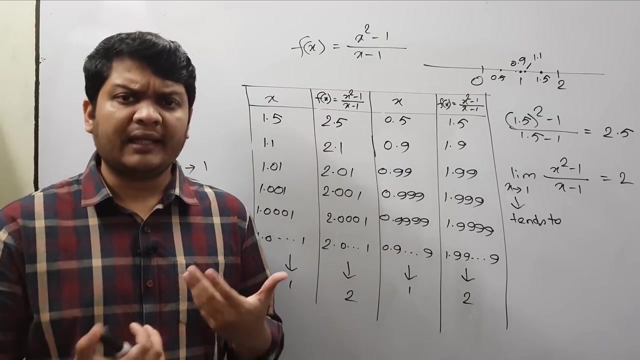 tends towards 1, then the value of the function, that is, the output of the function, will be equal to 2.. This is the concept of limit, But the good news is that we will not calculate each and every mathematical problems. in this way. We will have some knowledge about how to calculate the problems. 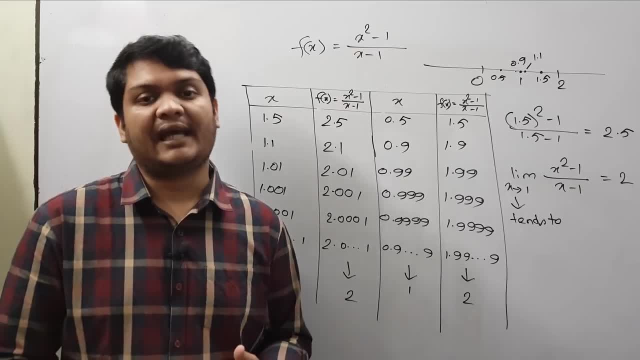 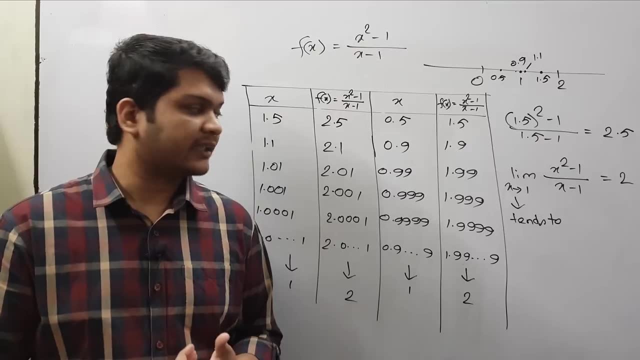 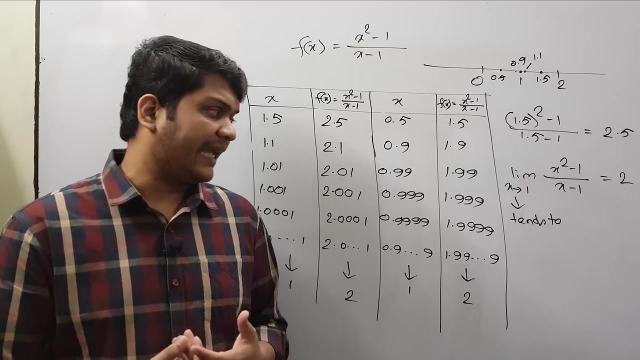 of limit And we will learn some different techniques and shortcut procedure to calculate the values of those functions in the later parts of the series, But today we have got some ideas about what limit is. So, in short, what is, if I say, the basic idea of limit is that when we are not being able to 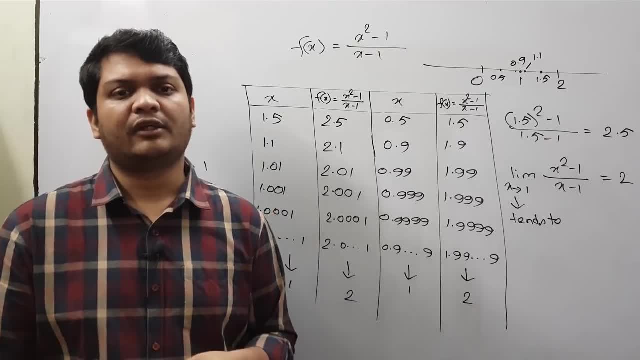 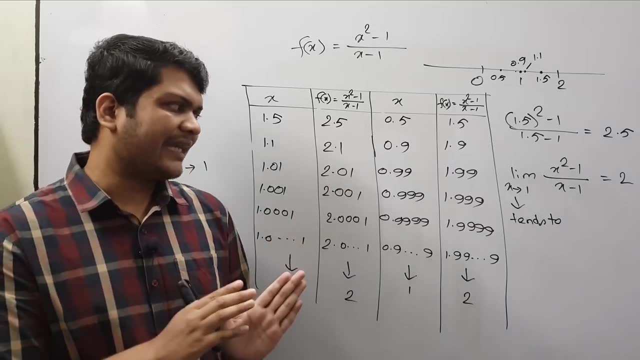 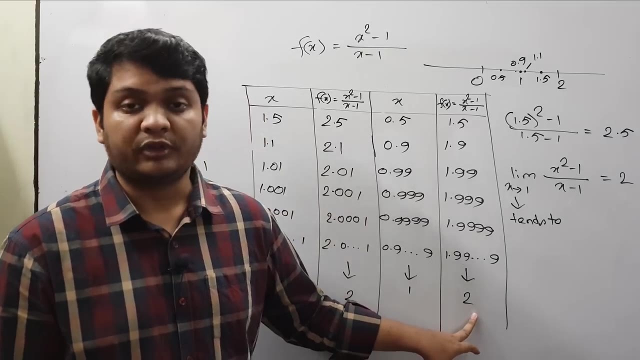 calculate the values of those functions directly. in those cases we try to put values which are much more closer to the input. we will decide that if we can move towards that particular value, then the result would be equal to the output which is approaching right. so this was the basic idea of limit. today we have discussed 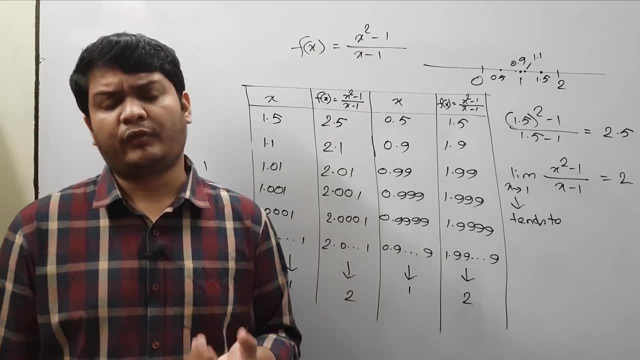 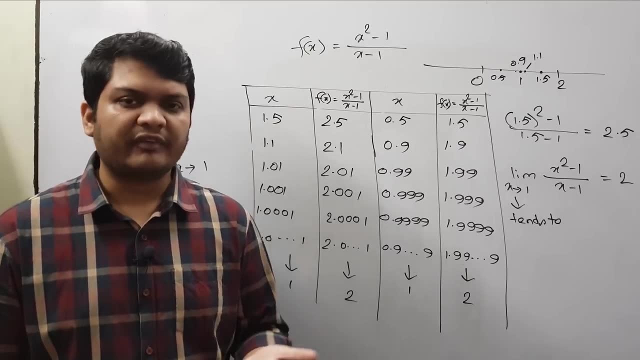 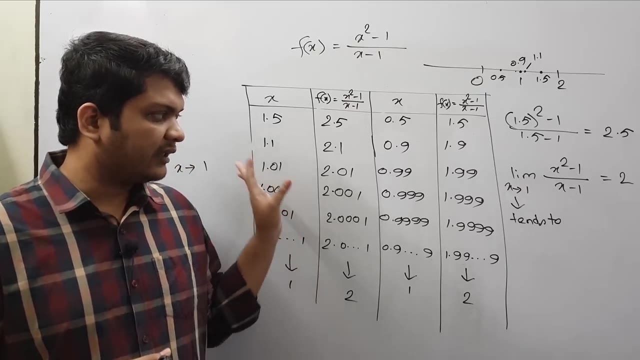 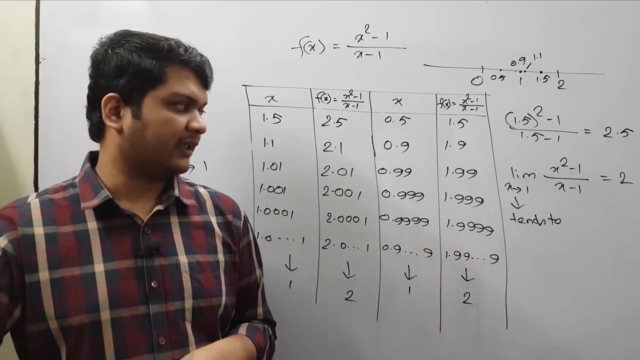 about uh, from the function with the conditions of functions, and then we have discussed about limit and in the later sections of the series, i mean from the next videos, we will be learning about the procedures and techniques, how to calculate limit, and we will not discuss in details that how we have approached towards that value. so will not take much time for each and 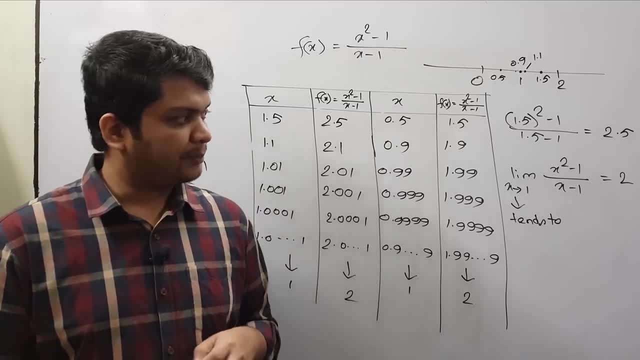 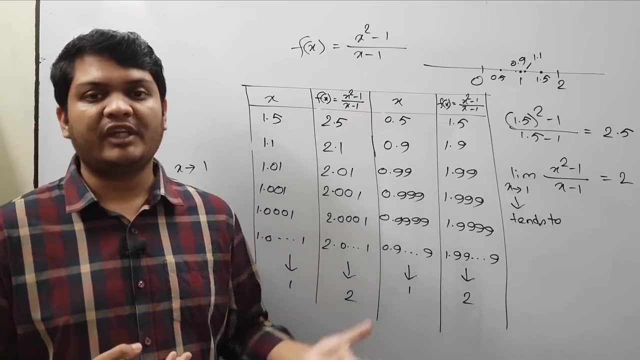 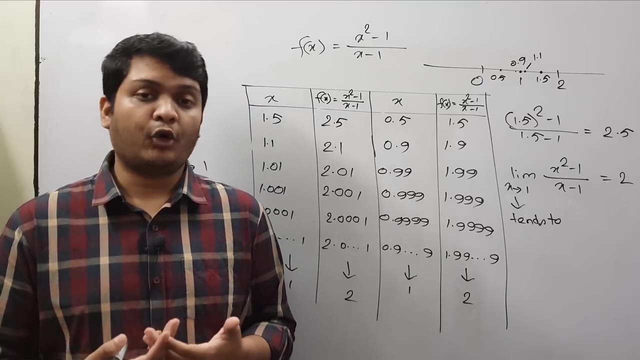 every problems in the later sections. so this was all for today's video and if you learned something, if you think that this video was helpful for you, please let your friends know about my channel and subscribe my channel, and i wish and i hope that you will be with me in the upcoming days, which will inspire me making 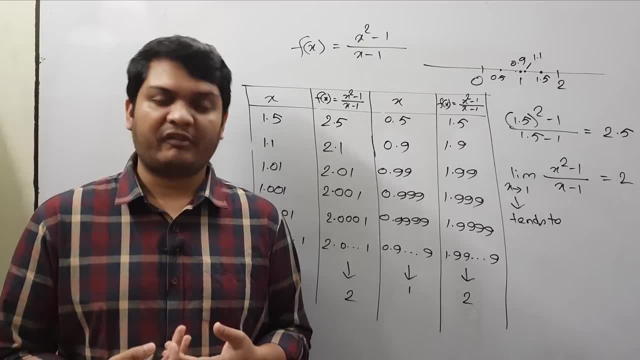 more videos. so till the next video. stay well, pray for me, i also pray for you. stay fine, allah hafiz.